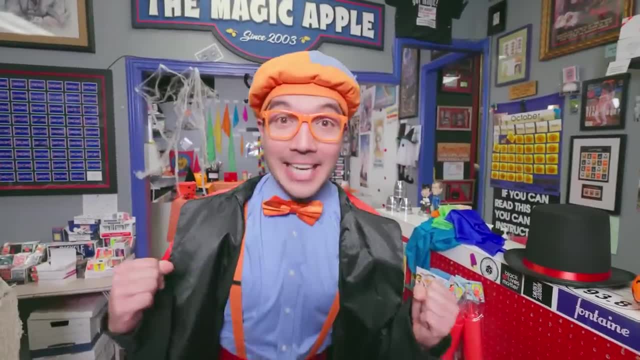 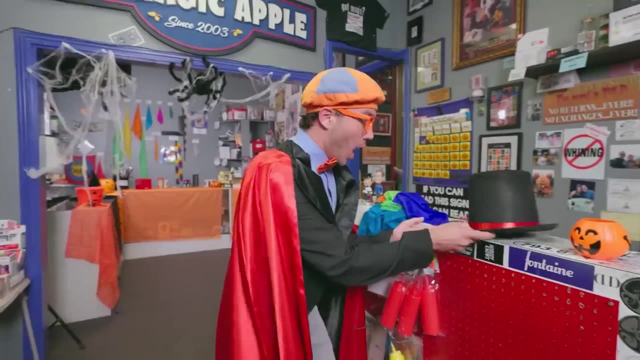 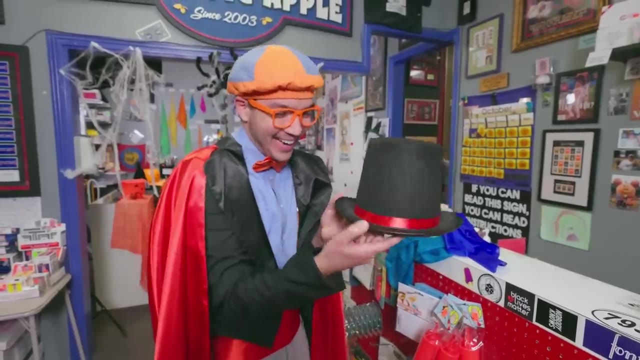 Whoa, I can't believe it. We're inside an actual magic shop And look at this. Do you know what this is? It's a magician's hat. Whoa, Maybe a rabbit will come out of this, Or something else. Maybe. I'll try that on later. 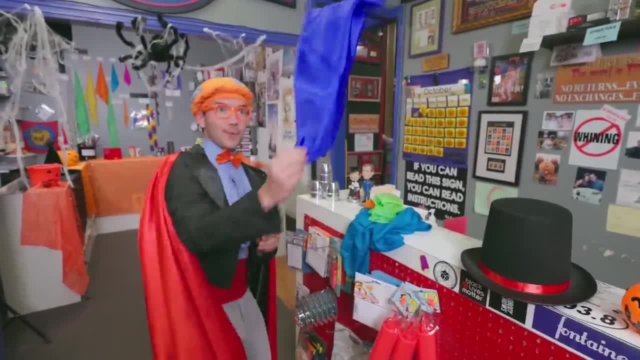 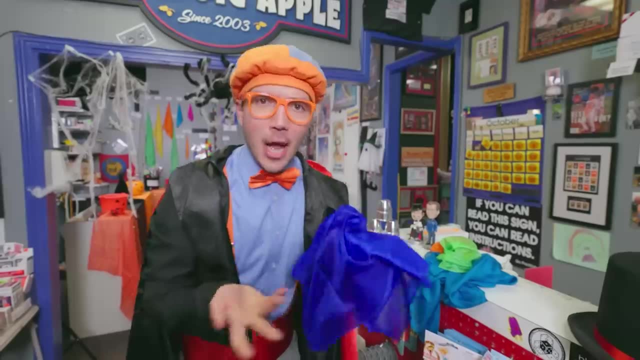 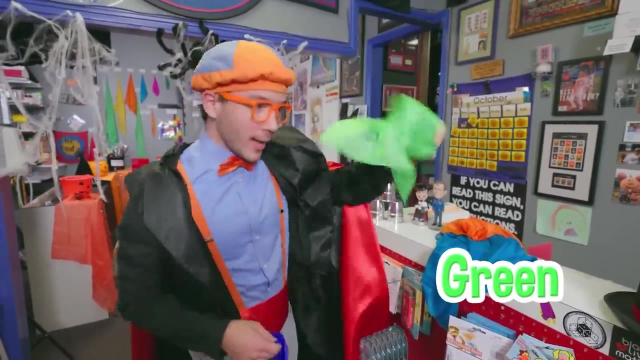 Oh, and look at this. Look, it's a blue scarf. Yeah, sometimes magicians use props. Yeah, those are things that help them do magic. Yeah, like a scarf. Woo, Whoa, There's a green one. 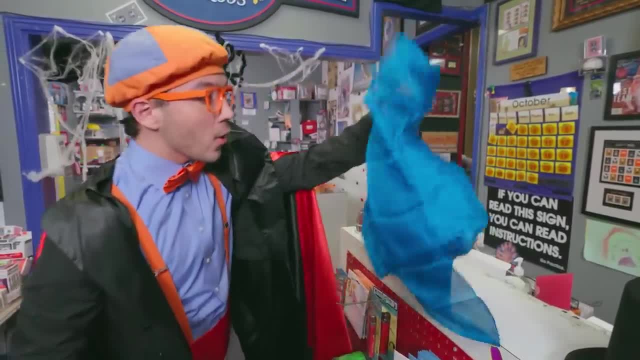 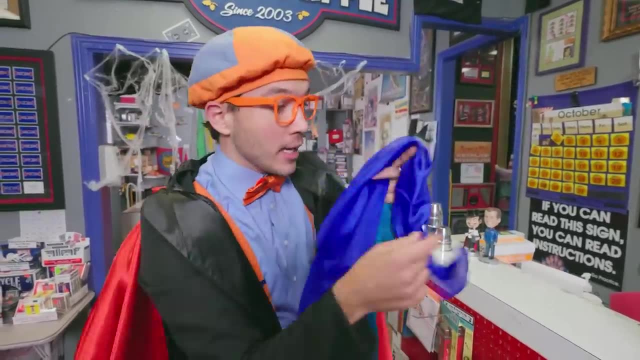 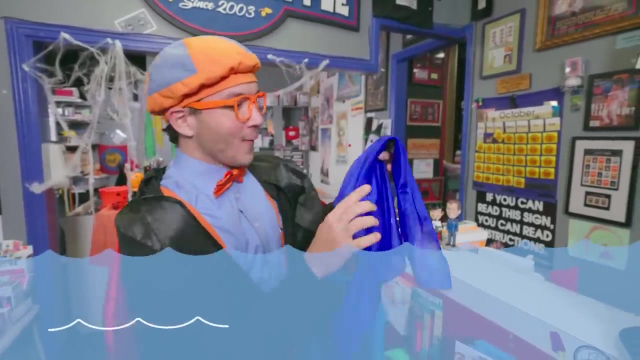 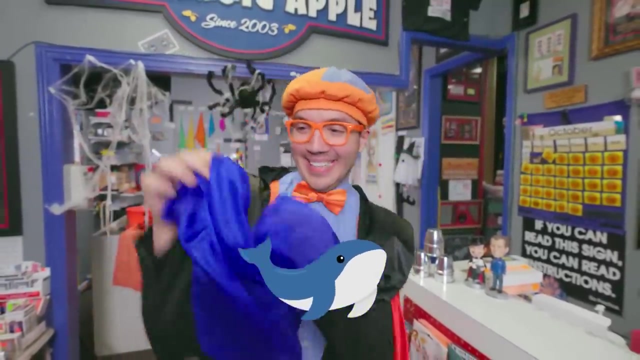 And an orange one, Whoa. And look at this, It's a light blue one, Whoa. Hey, Can you think of anything else that's also the color blue. Maybe the ocean. What else is blue? Oh, maybe a blue whale, Whoa. 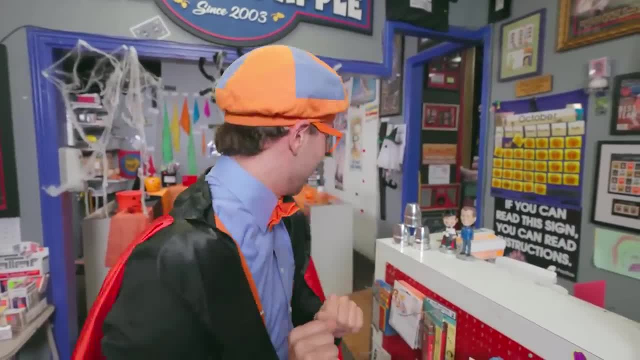 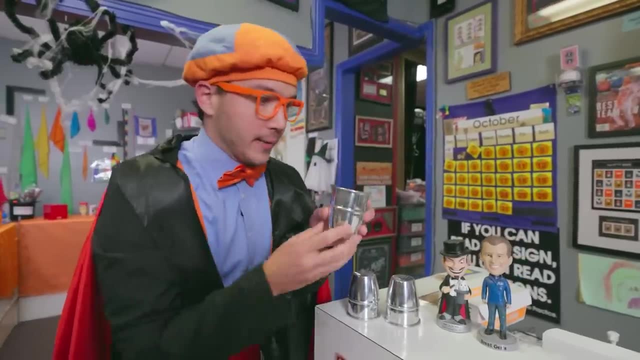 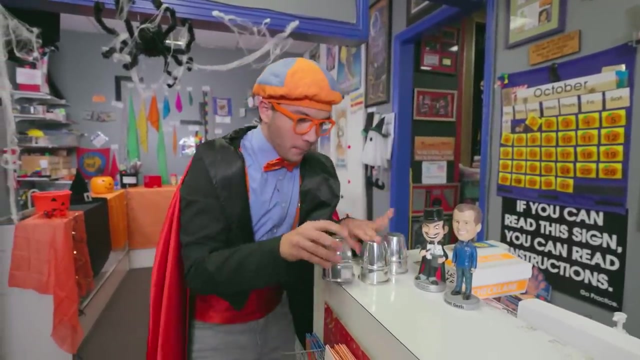 Well, let's see if we can find some other things here. Whoa, Whoa, check it out. Yeah, do you know what these are? They look just like a regular cup, But these are magic cups. Yeah, You can put things underneath them and rearrange them, and then they disappear. 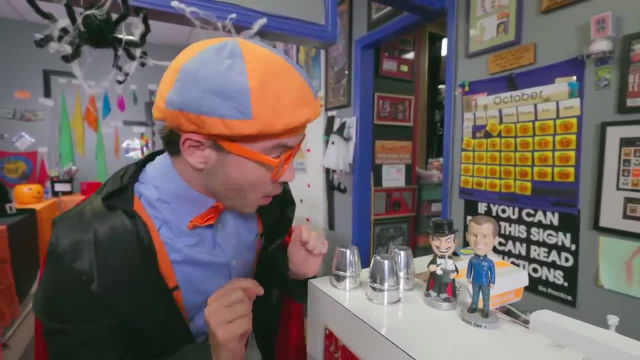 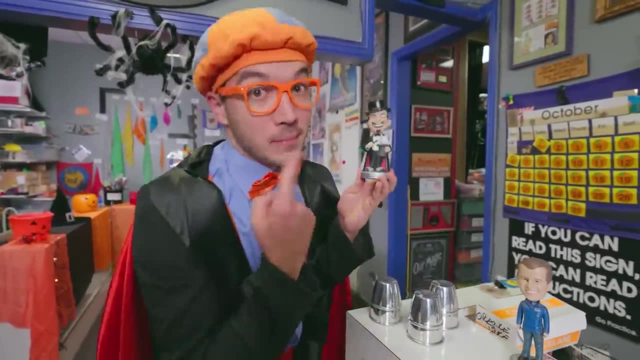 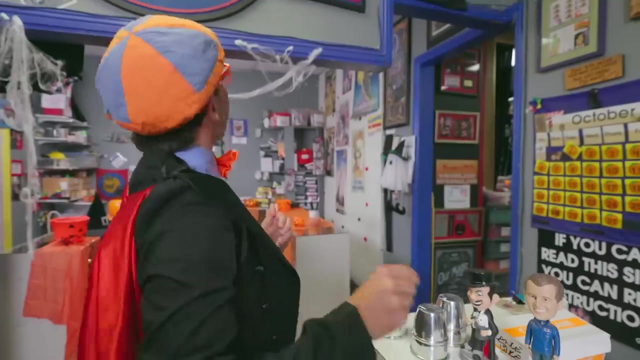 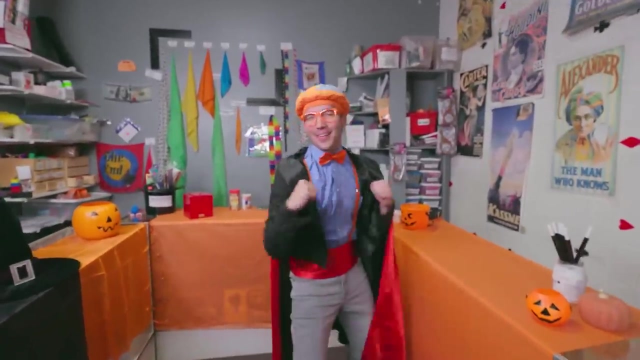 Or sometimes maybe they move spaces. Oh, hey, look, It's a little bobblehead. Yeah, well, this certainly looks like one cool magician. Yeah, I love dressing up for Halloween. Ooh Whoa. Yeah, it looks so cool here. Yeah, everyone is all ready for the holiday. 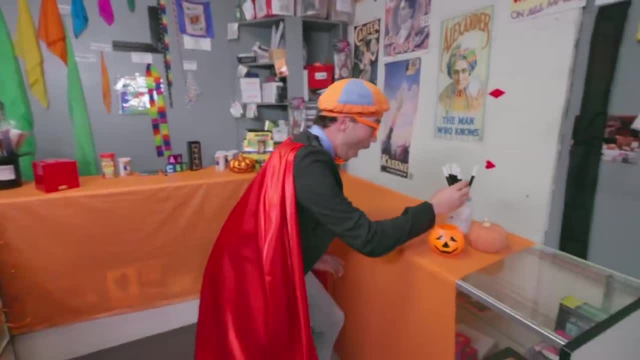 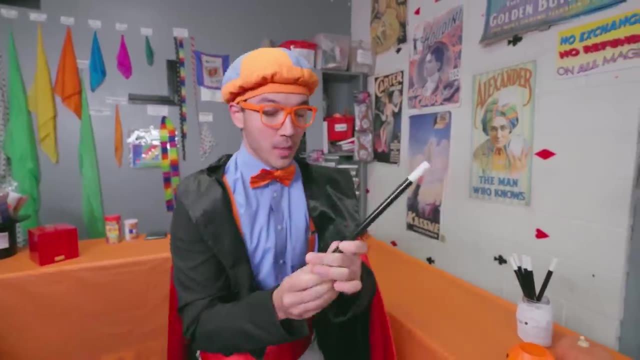 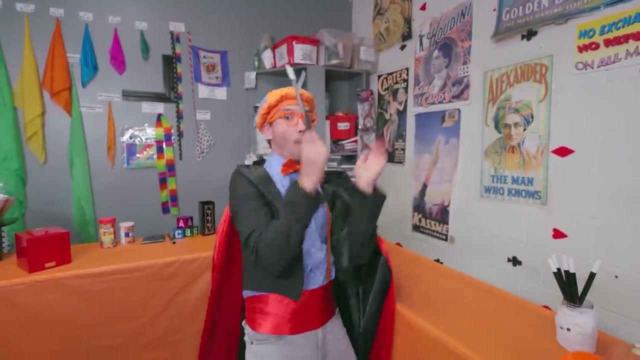 Hey, guess what's here? Oh, Whoa, Whoa, We found it. Yeah, The perfect addition to my costume. This is a magic wand. Whoa, Yeah, look at it. Yeah, the magic wand helps a magician do tricks. 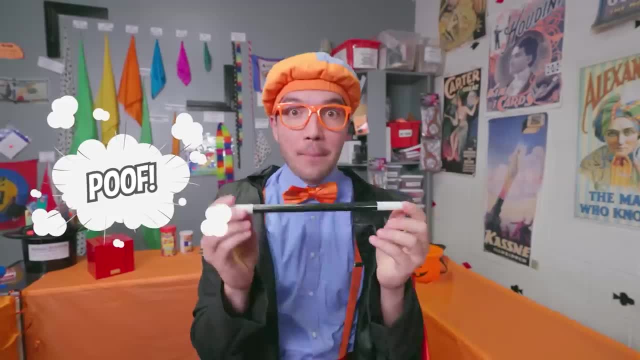 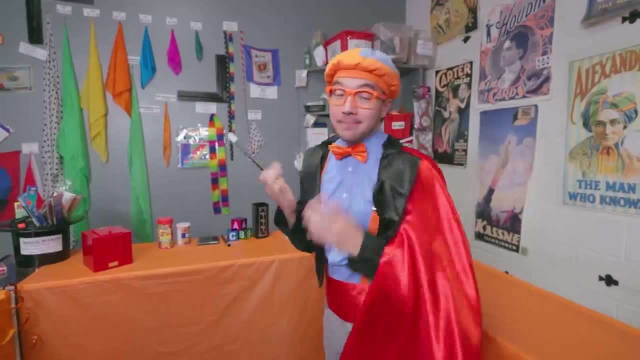 Kind of like the scarves or those magic cups. But this is the most important thing, Whoa, Hmm, Well, this is a lot of fun exploring the shop, but I think I need a little help to become a better magician. Yeah, 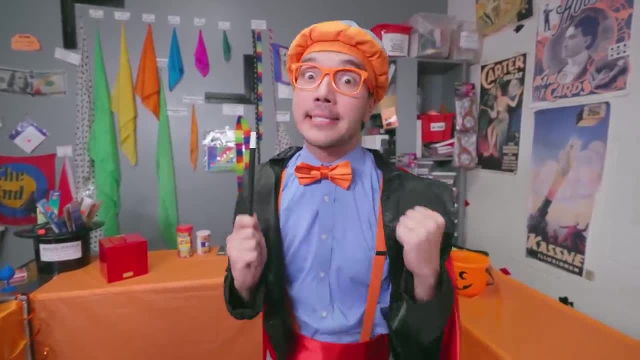 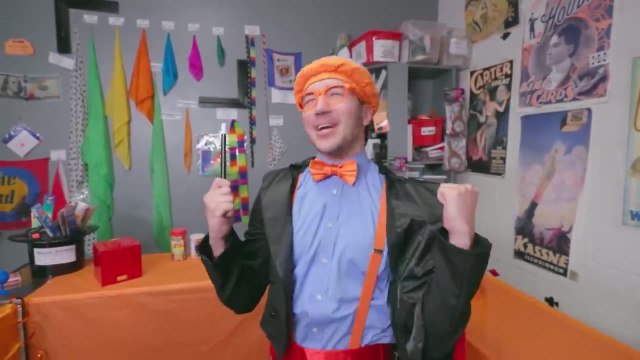 Magicians: yeah, all the tricks they do takes a lot of practice, And I think having a teacher would help me practice so I can do some amazing tricks for Halloween. Hmm, Ooh, maybe we can find one over here, Hmm. 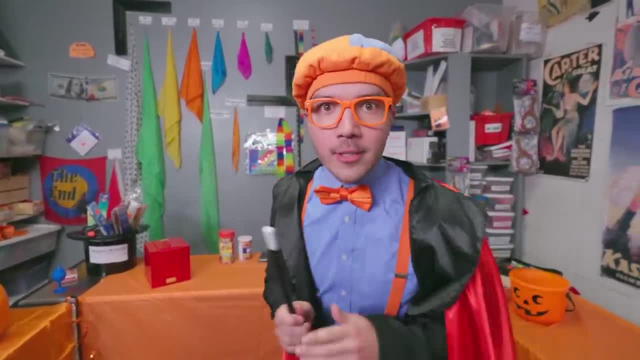 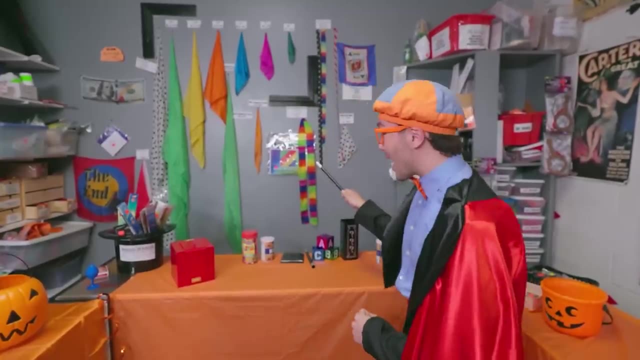 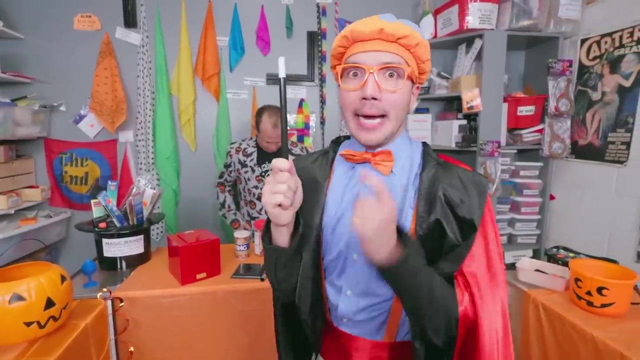 But first we need to say the magic words. Hmm, Ooh, I know the perfect magic words. Are you ready? Here we go. Silly potato, Whoa, Whoa. It actually worked. I think I'm going to put this down now. 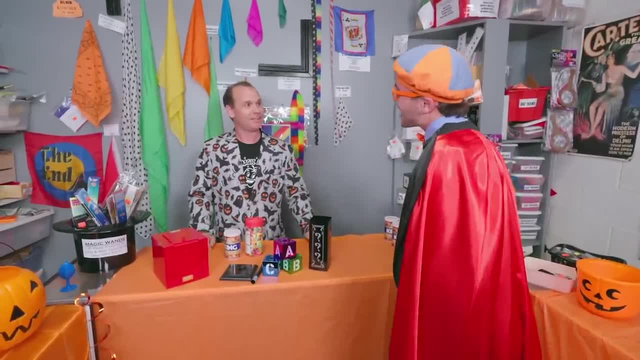 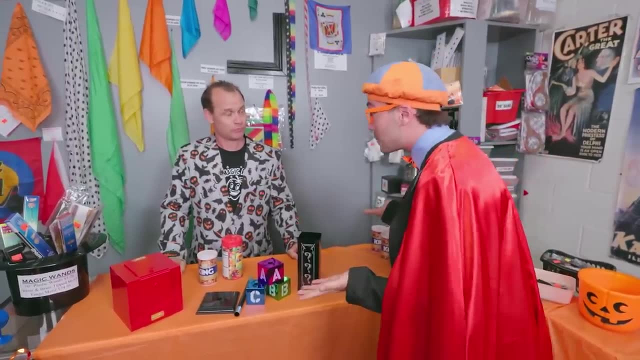 Ooh, let's say hi, Hello, I'm Blippi. What's your name? Hi, I'm Brent. Oh, it's nice to meet you, Brent. Well, I'm dressed up as a magician for Halloween And I was hoping to meet a magician so I could learn how to do some magic tricks. 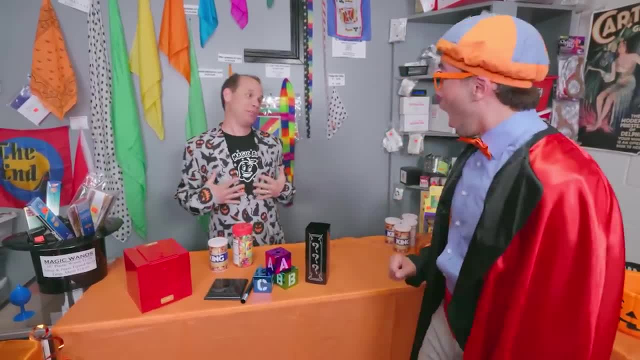 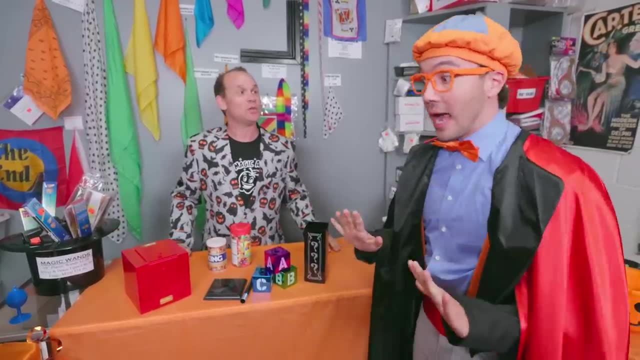 Do you know any magicians? Well, I'm a magician, Blippi, and I own this store. Whoa, You're a real-life magician. Yes, Whoa, That's awesome. Well, I want to be the best magician I can be for Halloween. 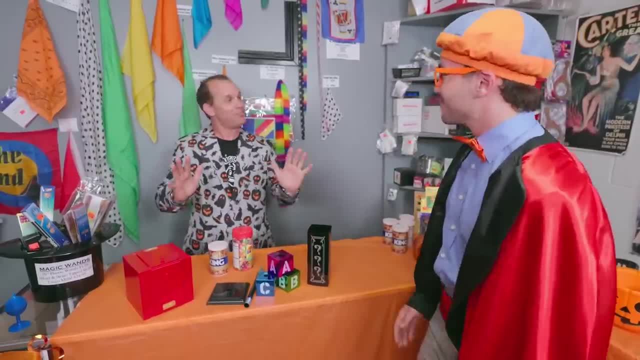 So do you think you could show us a trick? Sure, I thought, yeah, I definitely will. But before we start, I thought it'd be fun to have a little snack. So I have some jelly beans here, or deluxe mixed nuts. 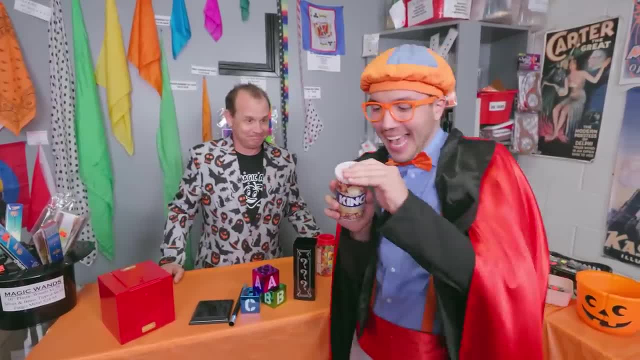 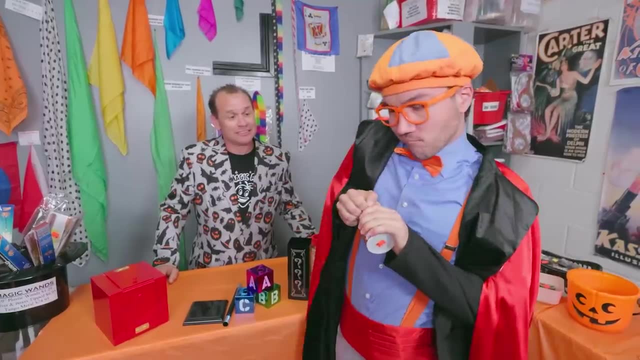 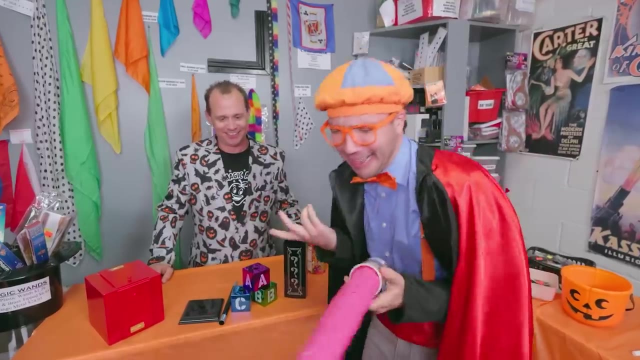 Which one would you like? Well, I can't wait to eat some yummy nuts. Yeah, cashews and almonds and all kinds of things. It's kind of stuck on there. Those aren't mixed nuts. Whoa, Those aren't mixed nuts either. 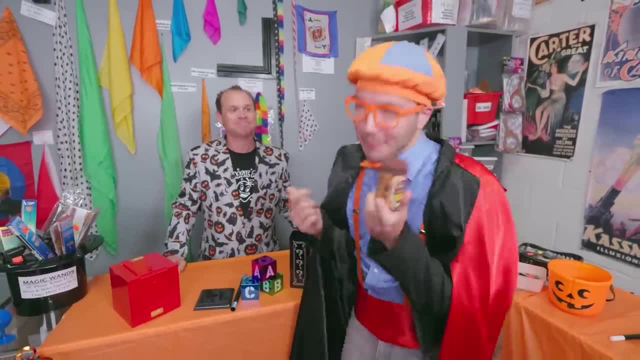 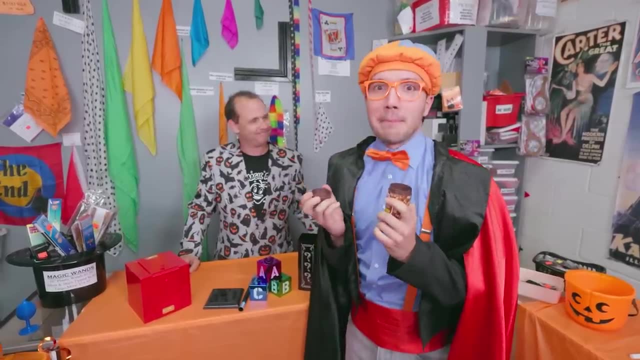 Well, I'm still kind of hungry for a snack. Good thing I brought some from home. OK, Mm salted mixed nuts. Ooh, these look so tasty. Maybe I'll have a snack later. Well, that was really fun. 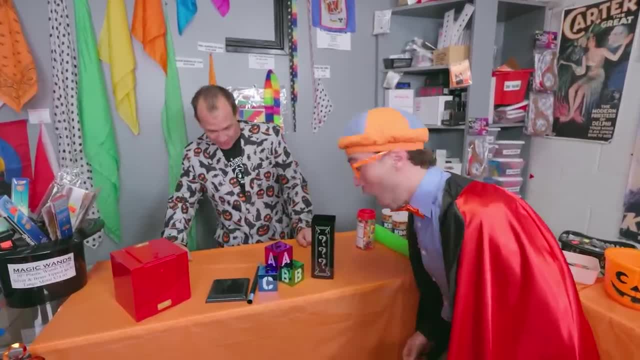 Oh, and what's this right here, Brent? Well, this is a little magic trick I thought I would show you. I've got a magic wand that we'll place right there, And I've got a block with the letter C on it. 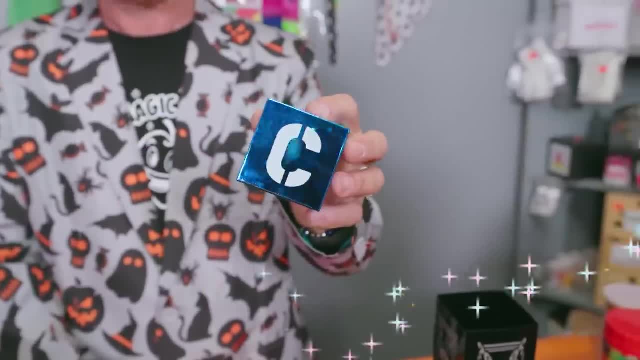 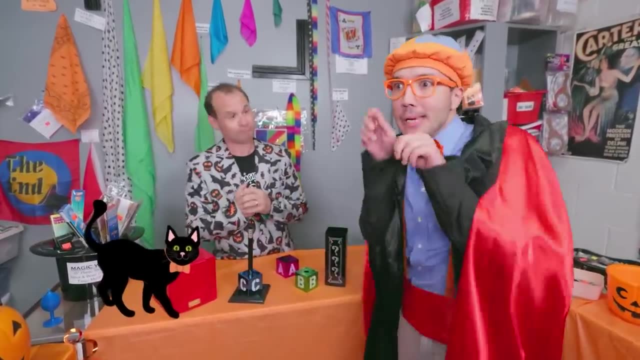 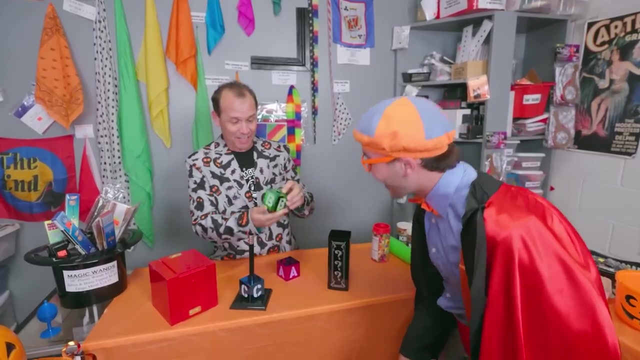 Whoa, It's a blue block with the letter C. Hey, can you think of a word that starts with the letter C? Hmm, maybe cat Meow, meow Or caterpillar, Ugh, And another one with the letter B. 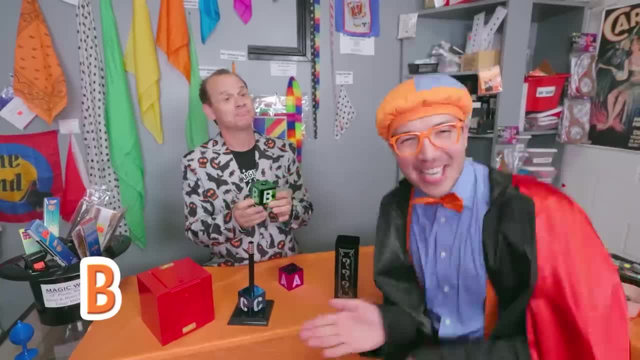 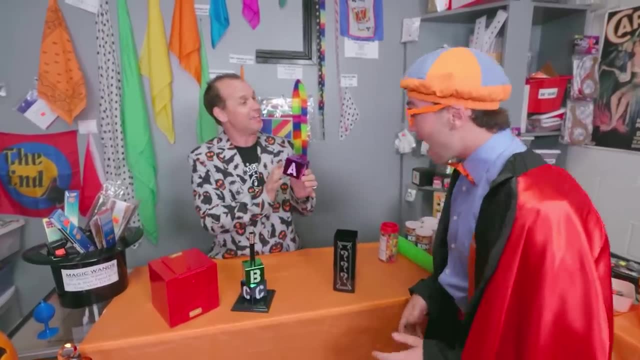 Oh, the letter B. Oh, just like Blippi. Oh, or Brent, That's right, I like that one. And of course, A, A, yeah, That's a really important letter. It's the first letter of the alphabet. 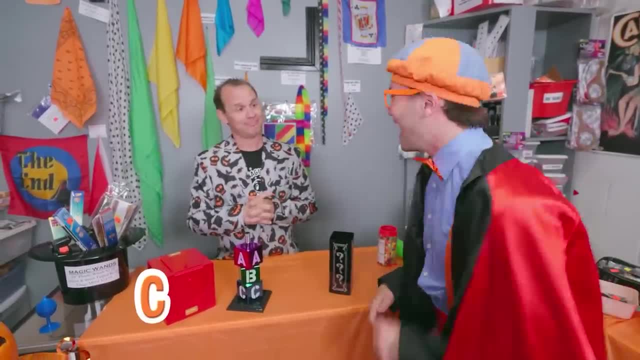 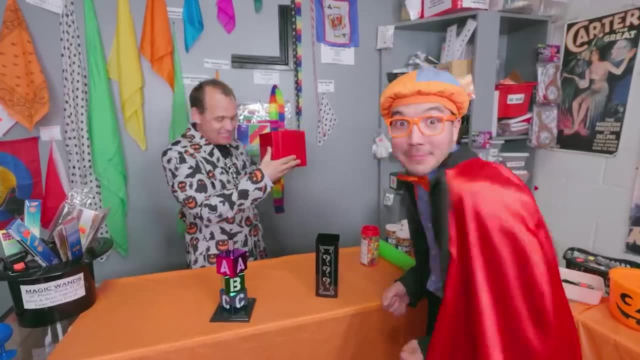 A, B, C And I have a very magical box here. Blippi, There's nothing inside the box here. Whoa, We'll use that in a second. And since your name starts with B and my name starts with B, 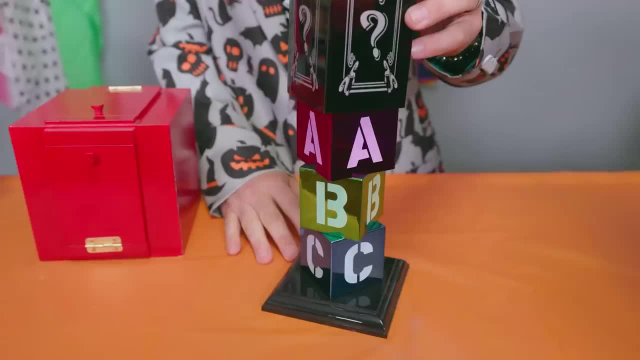 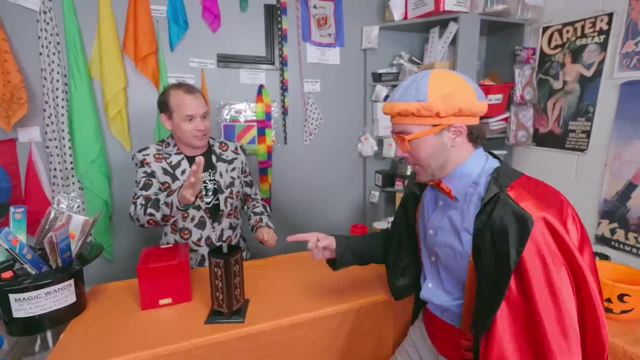 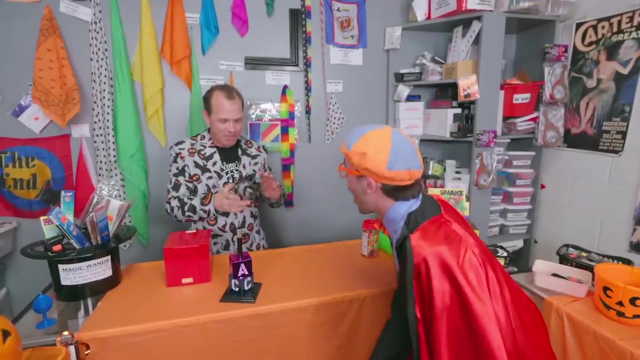 I'll show you this empty tube. Keep your eye on that green block. Do you know any magic words? Hmm, I sure do. Blippity, dippity, hop. Look at this. Whoa, The B disappears. Whoa, check it out. 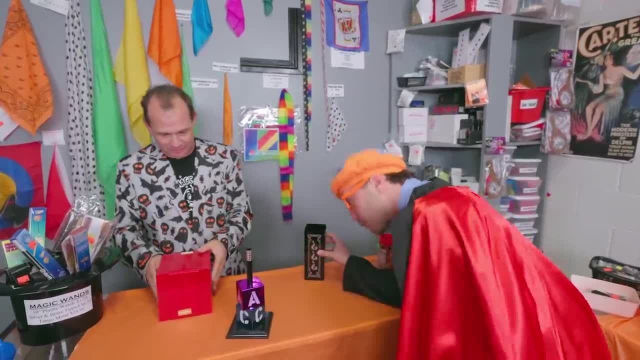 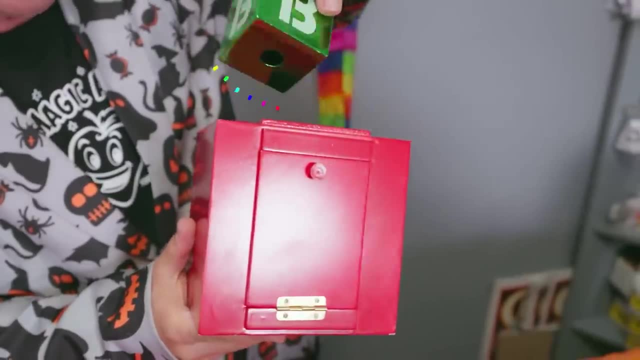 Hello, Huh, there's nothing in here. Whoa, where'd it go? Leave my empty box? Yep, it has a little magic bee. Whoa, yeah, that was awesome. Whoa, Brent, you're an amazing magician. 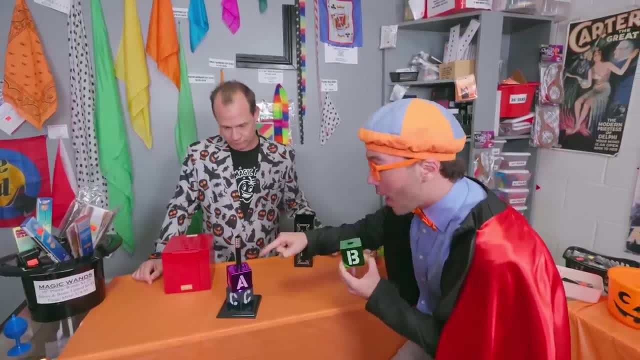 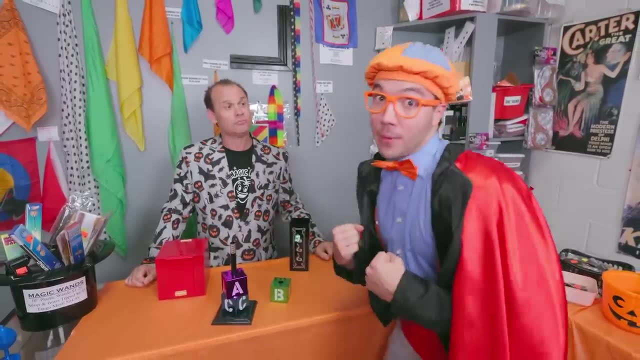 Whoa, he moves the bee from the magic wand into the box with magic. Well, that was so fun. Well, I'm already starting to feel like a real magician. Do you think you could show me another trick? Sure, let's learn a new trick and I'll teach it to you. 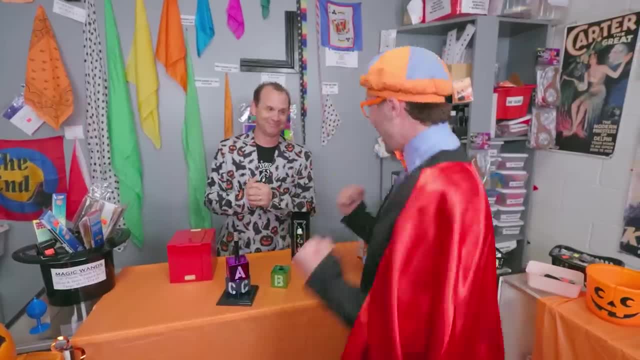 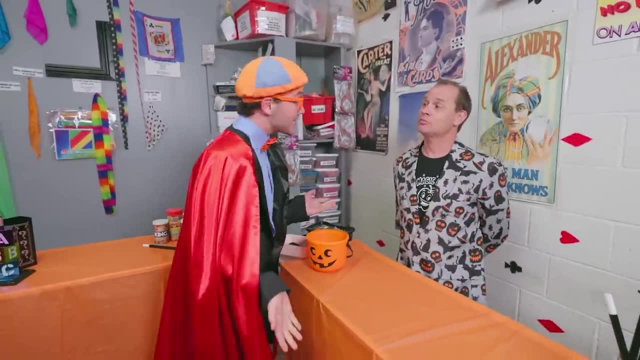 Whoa, I get to learn a trick on my own. Yeah, let's do it. Whoa, now we get to learn trick number two. So, Brent, what is this trick? Well, this one's a coin trick, and it's called close-up magic. 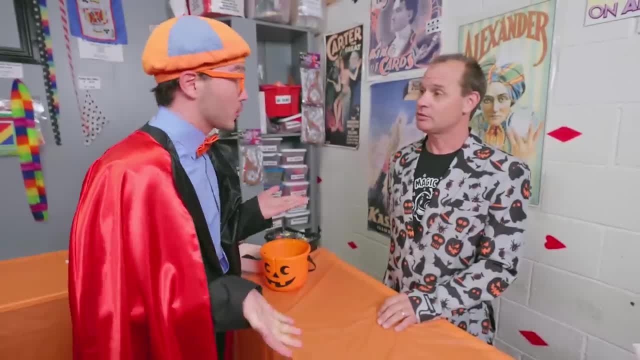 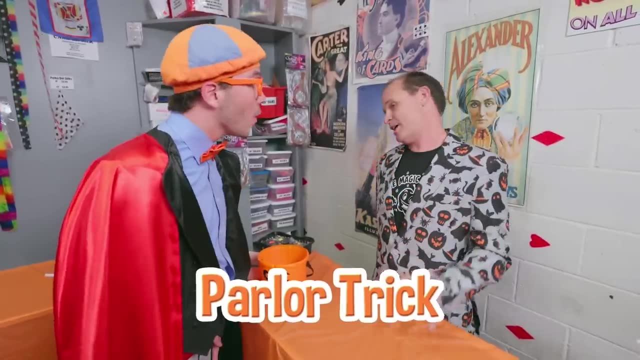 Close-up magic. Is that because you're really close to someone? Yeah, some things are smaller, like a coin trick is smaller than the trick we did over there, which is a parlor magic trick. Whoa, so it's a little bit bigger. 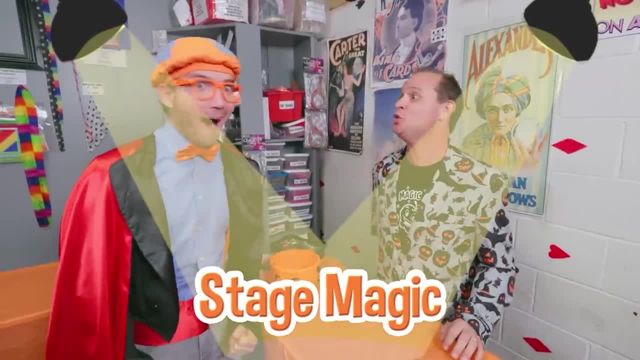 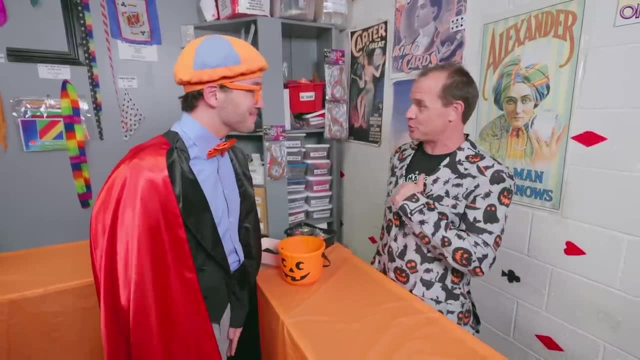 Yeah, exactly. and then there's also stage magic where they do illusions, Whoa, and I bet that's really fun, Really really big, It's huge stuff. so let's do a close-up magic trick for you and your friends. 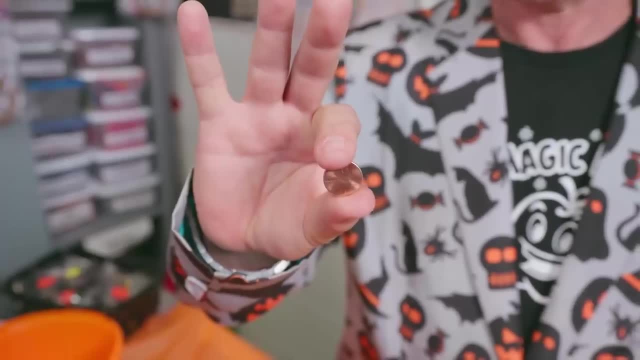 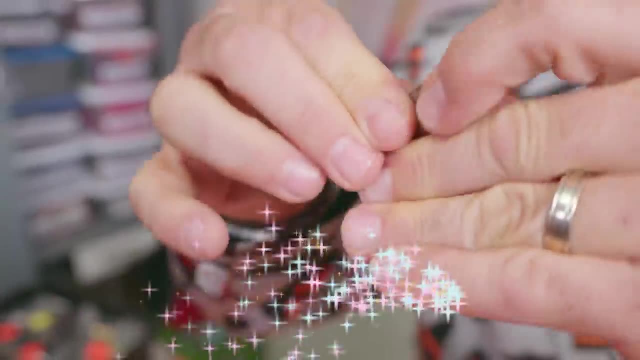 Okay, let's watch. I have one penny here and if you watch really closely you can't buy a lot of stuff with a penny. With a little bit of magic I can do this, hopefully, and then have two quarters. 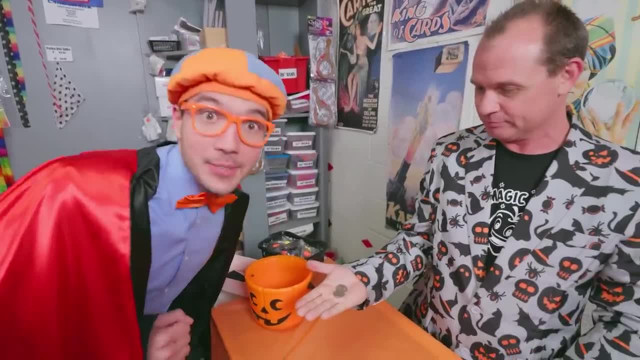 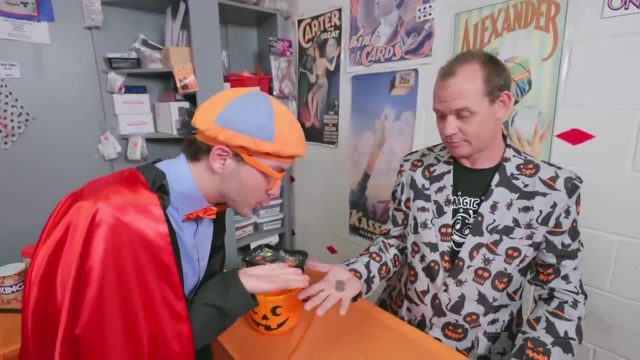 just like that, from one penny to two quarters. Whoa, that was amazing. Did you see that? Yeah, there was just one penny, Just one cent, and then it turned into two quarters. Whoa, two quarters, 50 cents. 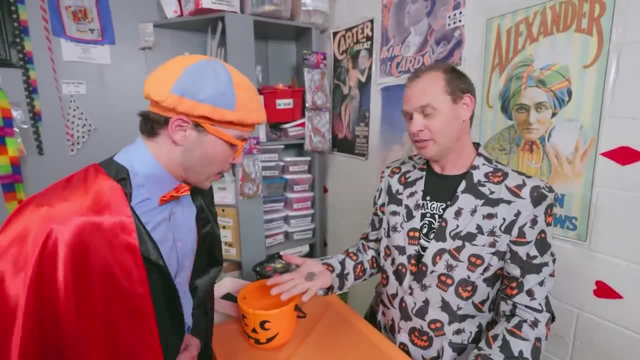 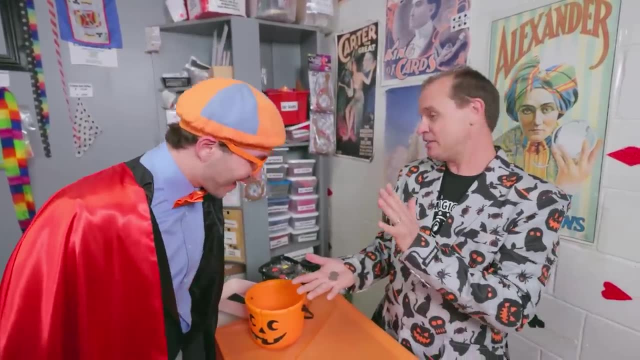 That's a lot of cents. Do you want to learn that magic trick? Mm-hmm, yeah, Okay, Definitely would like to learn it so that it makes a little more sense. So you have to promise not to tell the secrets of the magic trick. 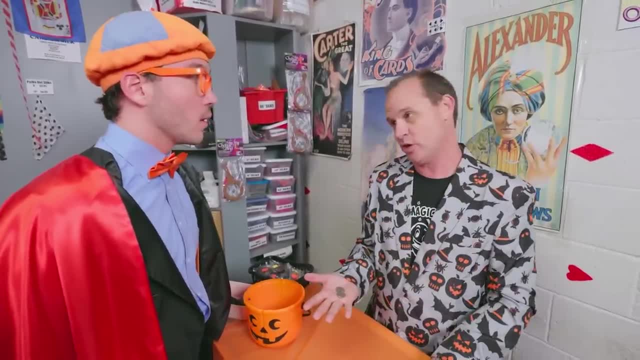 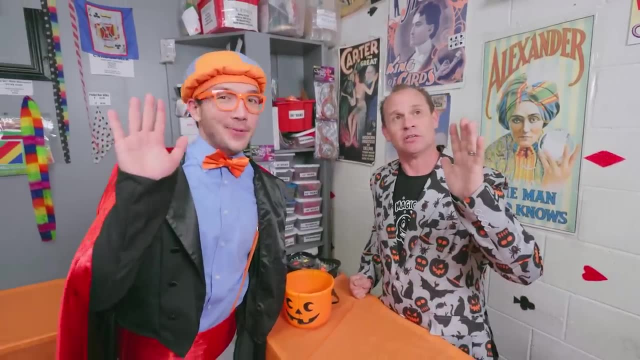 That's what makes a good magician, is not telling how the trick works. Oh well, I want to be a really good magician, so, yeah, Okay. so raise the hand that you write with Okay, Say I promise, I promise. 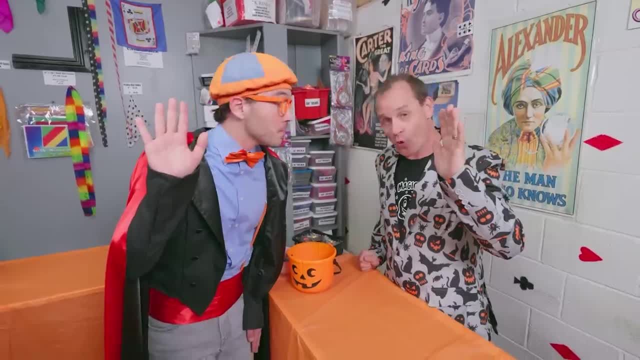 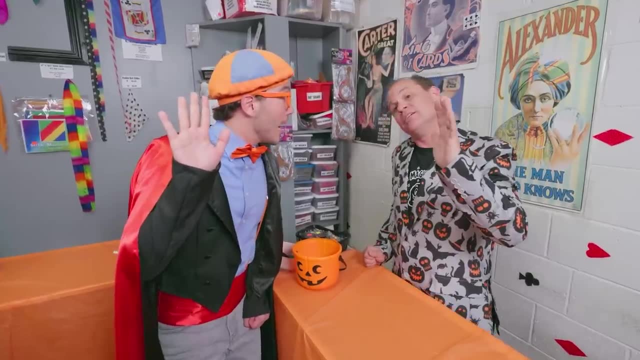 Not to tell the secrets, Not to tell the secrets Of the coin trick, Of the coin trick. And if I do tell the secrets, And if I do tell the secrets, Then I will be in. I will be in Big. 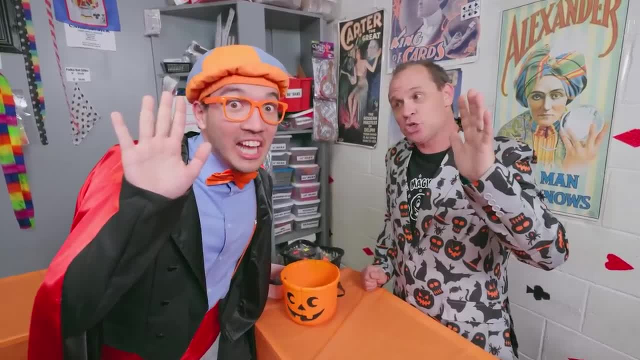 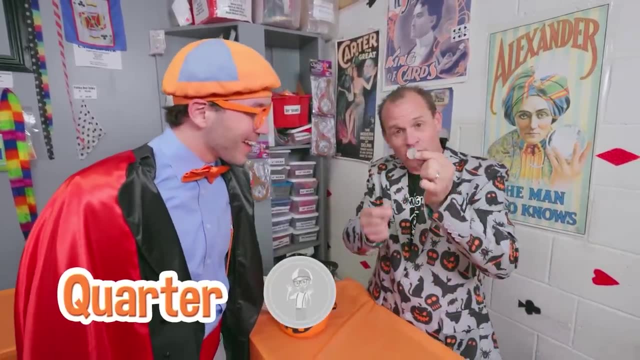 Big, Big, Big Trouble, Trouble. I don't want to be in trouble. So what you're going to need, Blippi, is you're going to need a quarter, Okay, And then another quarter, Oh, And then a penny. 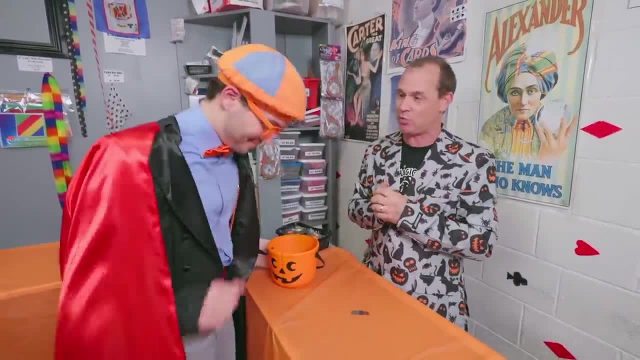 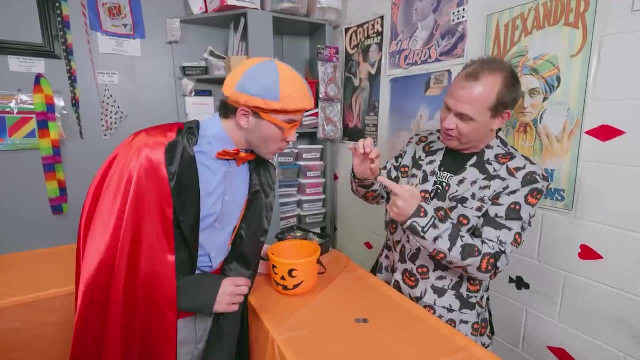 Okay, You need those three items to make this trick work. Okay, So before you start your magic trick, you're going to put the penny in between your first finger and your thumb, Ooh, And then behind that penny, kind of like a T. 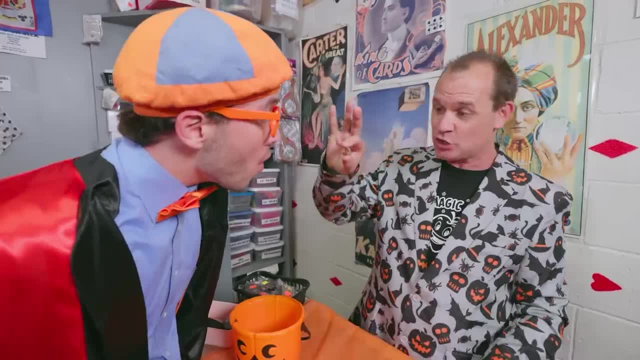 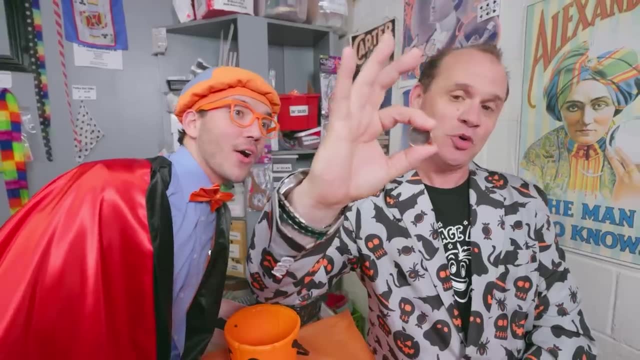 the two quarters go like that. So from the front of the coin it looks like there's one penny, But from the side there's two quarters Whoa. So you're going to be careful to watch your angles, Mm. 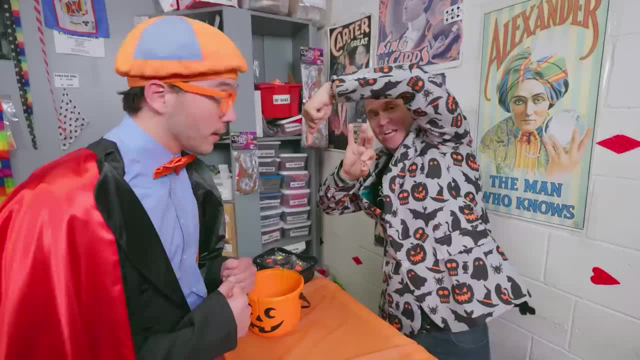 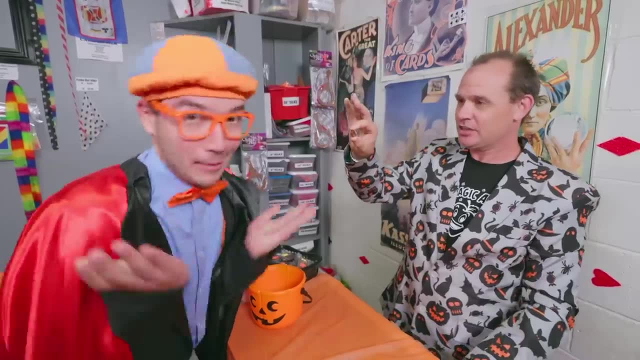 Yeah, To make sure nobody's on this side of you or on this side of you, but straight on, like you are. Whoa, Yeah, So the quarters are hiding in the back. They're hiding in the back, Exactly Yeah. 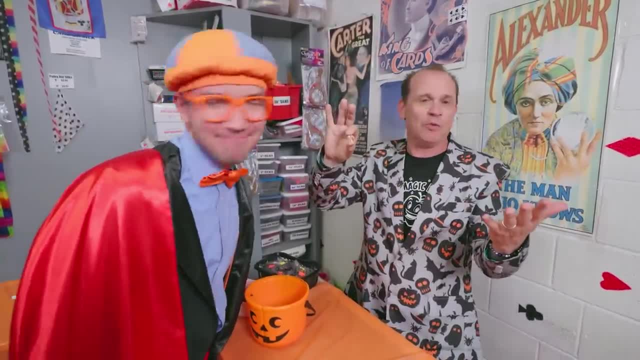 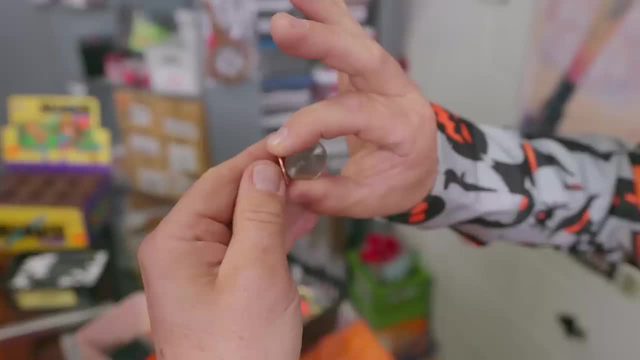 You can't see them. So you say to your friend: look, I have one penny, There's not much you can buy with one penny. And then when you cover up the penny with your hand, just like that, you're going to secretly push this penny behind the two quarters. 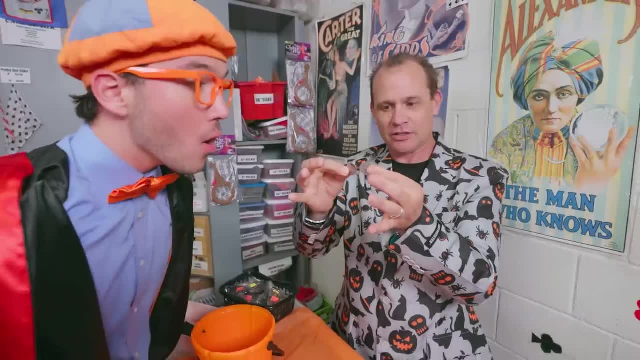 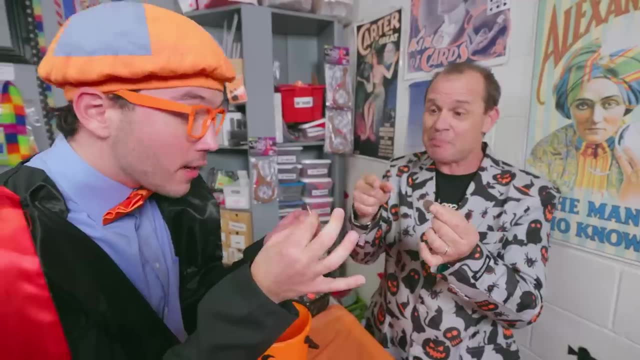 and show the two quarters. Whoa, That's amazing. Yeah, look, The penny is hiding behind one of the quarters Because the penny is smaller than the quarter. Oh yeah, See A teeny tiny penny, but a little bit bigger quarter. 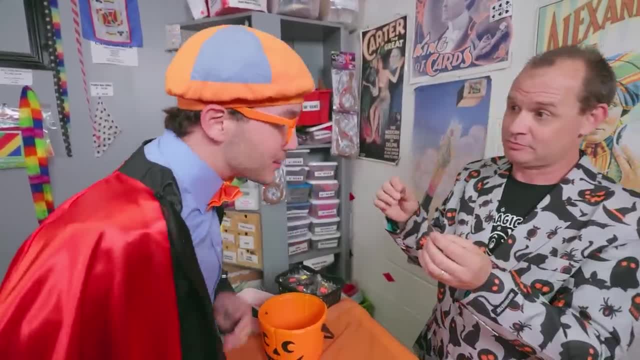 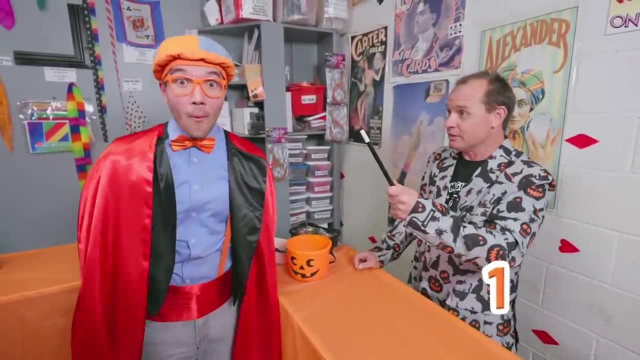 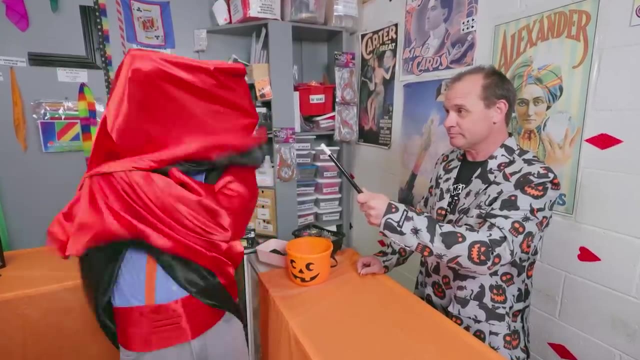 Whoa, Oh Brent, that's an amazing illusion. So now you've learned a magic trick, You're on your way to becoming a magician. I can't wait. One, two, three, I can still see you, Flippy. 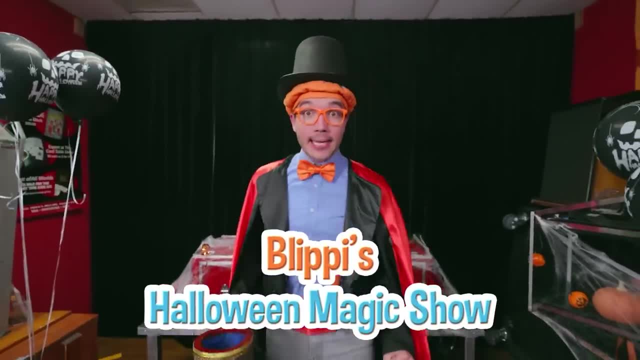 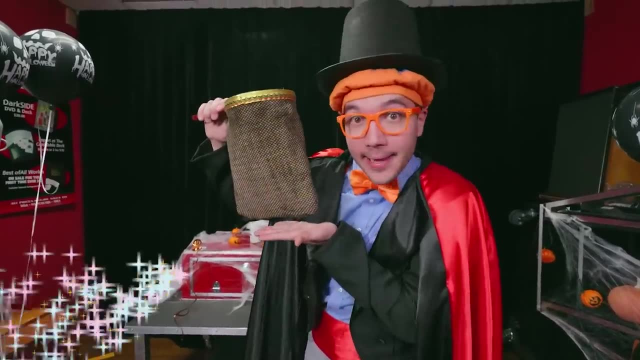 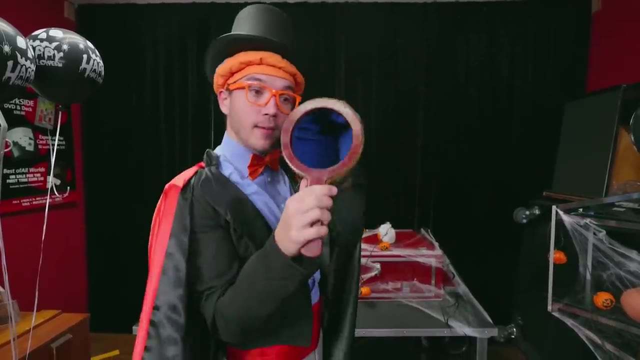 Welcome to Flippy's Halloween Magic Show, And now it's time for the grand finale. Whoa, Check it out. This is a magic bag. Yeah, This bag, it makes people forget things. Oh and look, There's nothing inside. 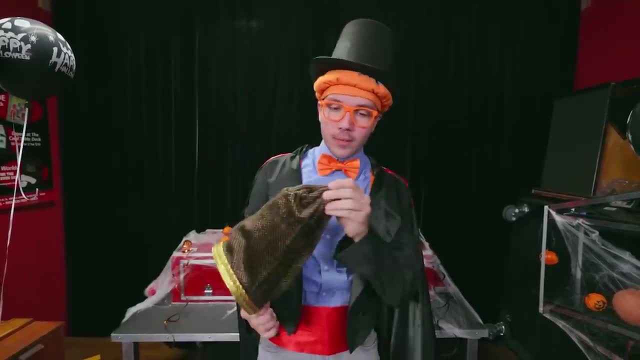 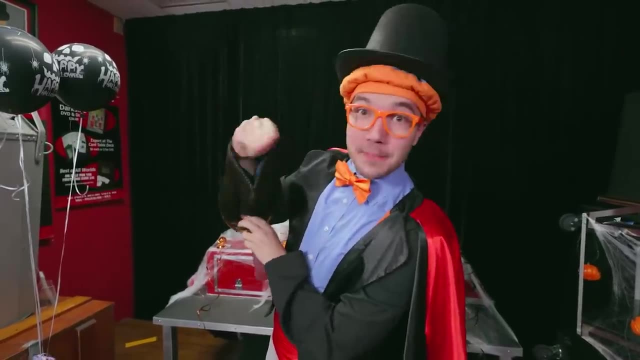 Nothing there, Nothing there. Oh, look, There's even a little zipper to show there's nothing inside, See, Oh, just my hand. Hello, Oh, hi there. How are you today, Flippy? Oh, I'm having fun doing a magic show on Halloween. 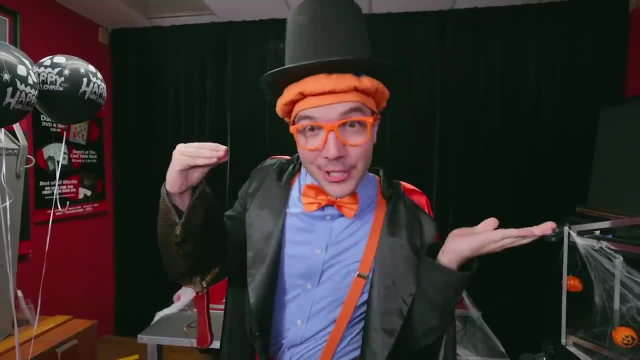 See you later. Bye-bye, Remember this bag? yeah, it makes people forget things, Yeah, So forgetful. Let's close up this zipper. Oh, and look at what I have here. Whoa, Look, It's a magic bag. 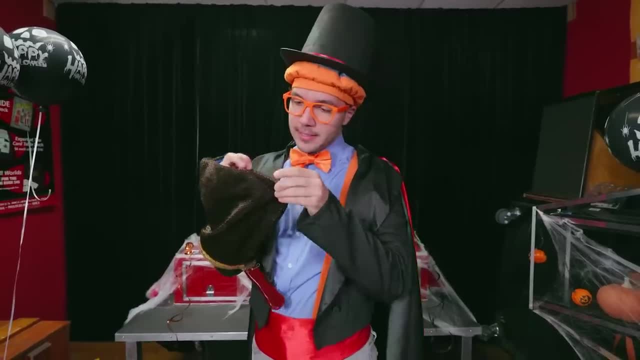 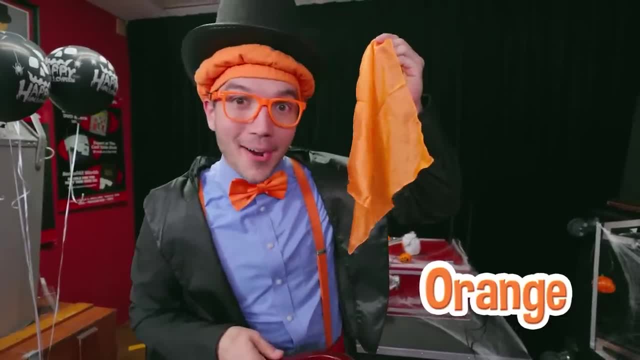 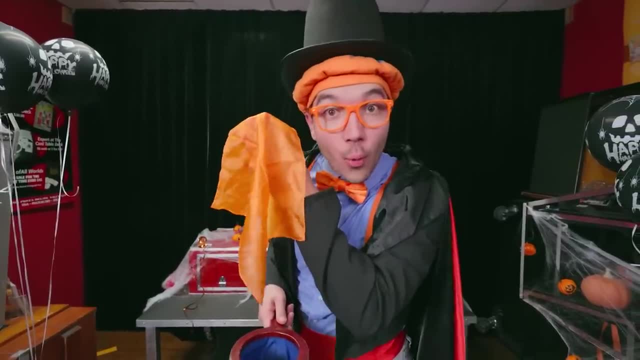 It's a magic bag. Look, It's an orange silk scarf. Yeah, orange, because orange is one of my two favorite colors. Whoa Hey, can you think of things that are the color orange? Hmm, Well, a fruit is the color orange. 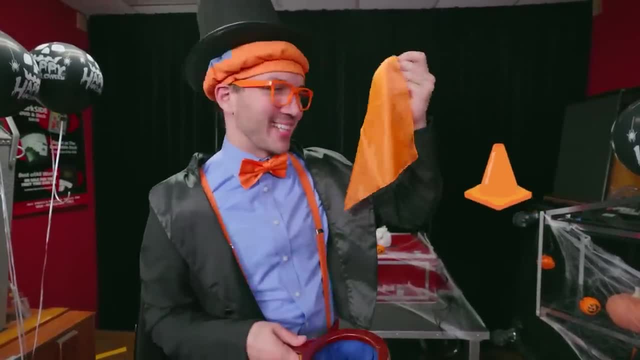 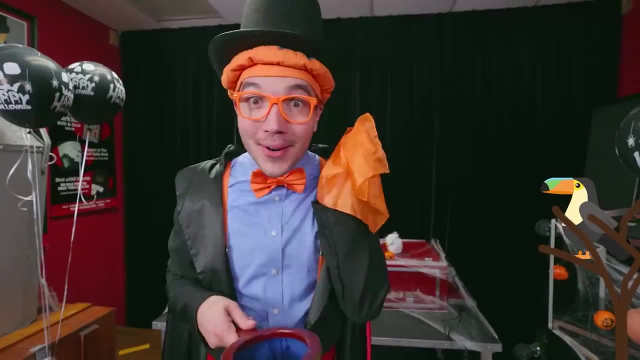 A safety cone. Yeah, That's also the color orange. Hmm, What else is the color orange? Ooh, Maybe a tropical bird. Okay, Well, let's put this orange handkerchief scarf into the bag. 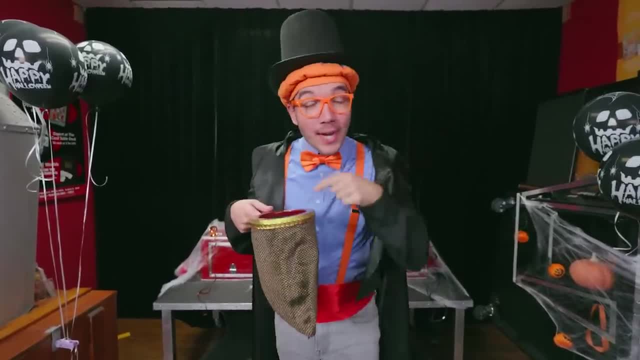 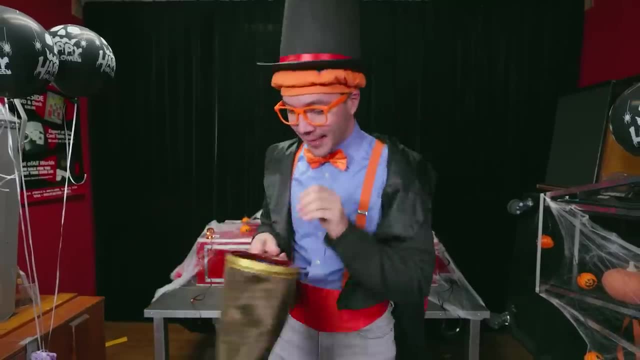 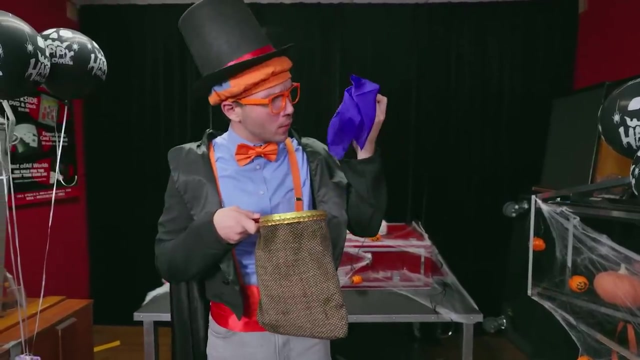 Wait a minute. the bag made me forget What color was the scarf again. Hmm, Oh, that's right, it was orange. Okay, you see, when you put it. wait a minute, I could have sworn. I put an orange scarf in there. 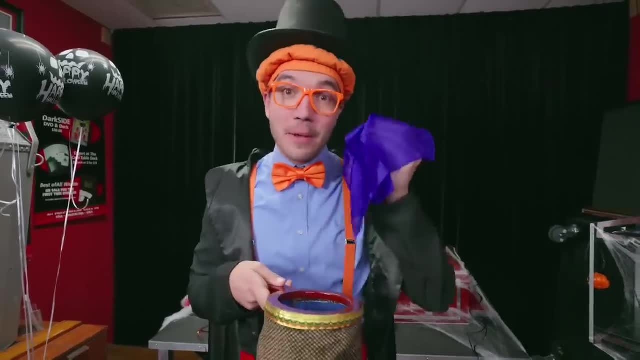 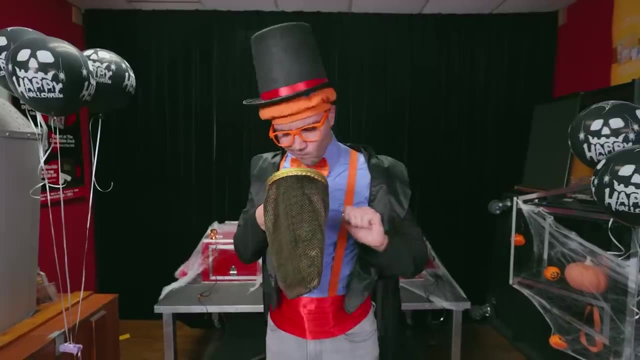 and now it's the color blue. Well, maybe if I put this blue scarf in it it will go back to orange. Here we go, It still looks blue to me. Well, maybe we need a magic word and it will go back to orange. 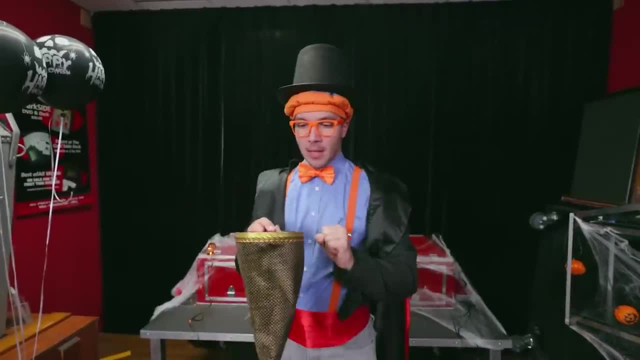 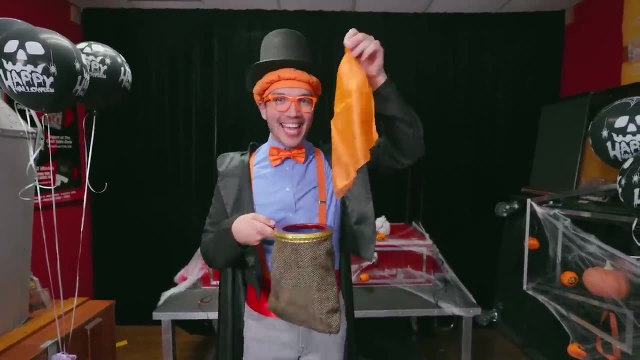 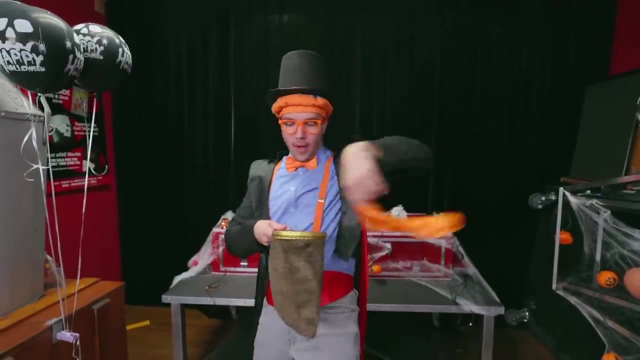 Can you think of a magic word with me? Okay, abracadabra. ooh, hey, it worked. Yeah, it's the color orange. Ooh, let's try turning it blue again. Okay, here we go. Whoa. 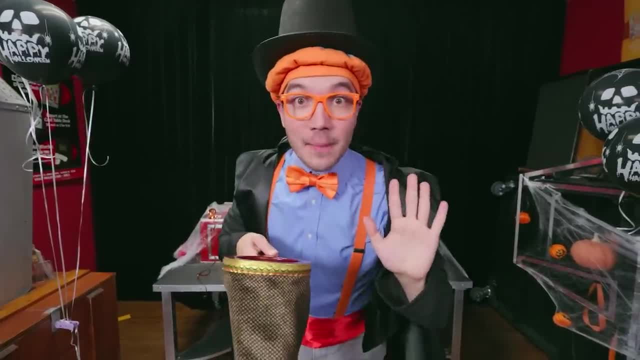 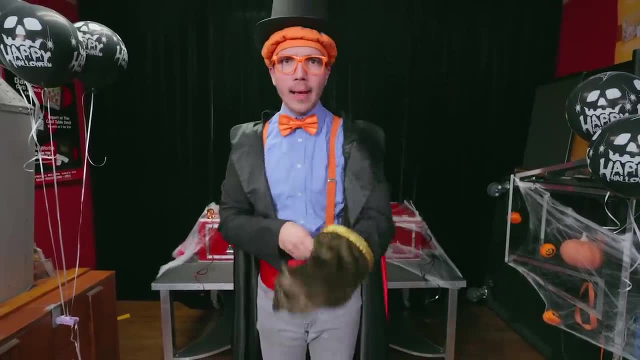 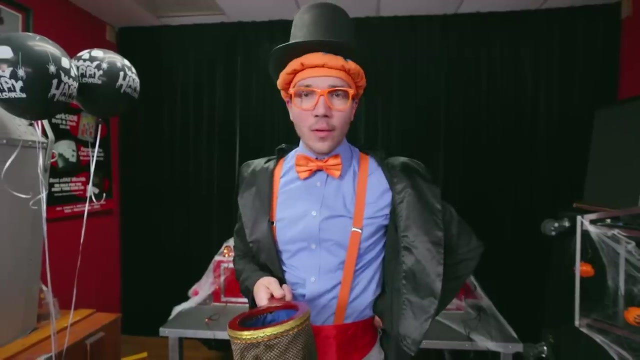 Are you ready to say the magic word to turn it blue? Okay, Silly potato. Wait a minute, there's nothing inside. Oh no, they went away. I wonder where their scarves went. Oh, I think I feel something. 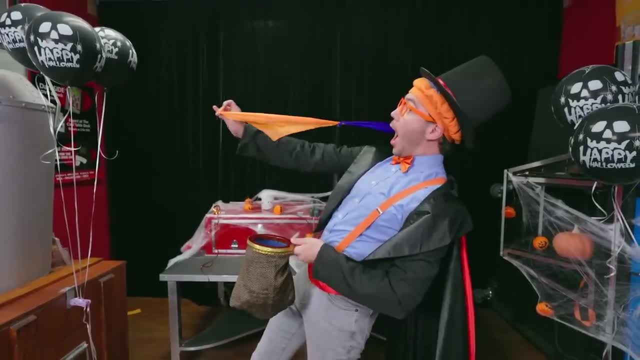 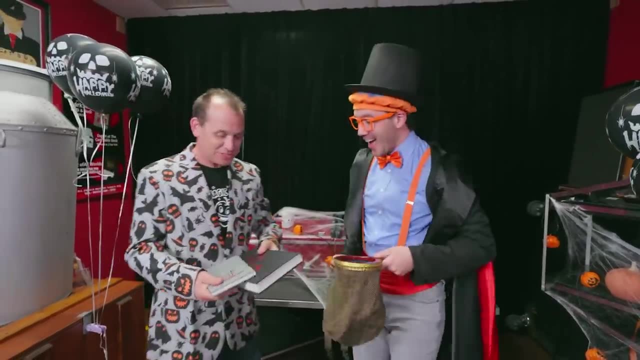 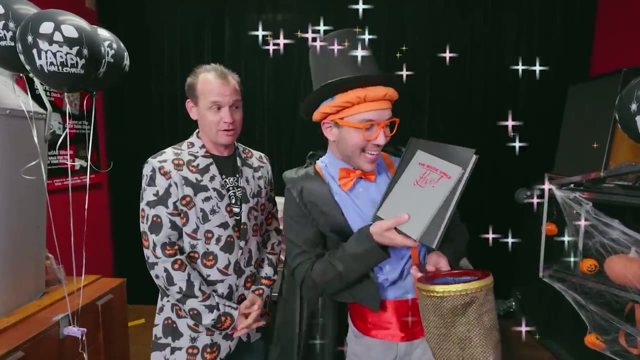 Whoa, It was in my ear the whole time. That was a great job. Bleepy, Give me a high five. and I brought some magic books just for you so you can keep learning more and more magic. Whoa, check it out- magic books. 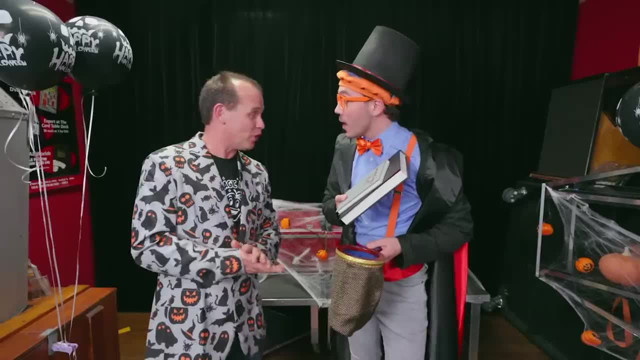 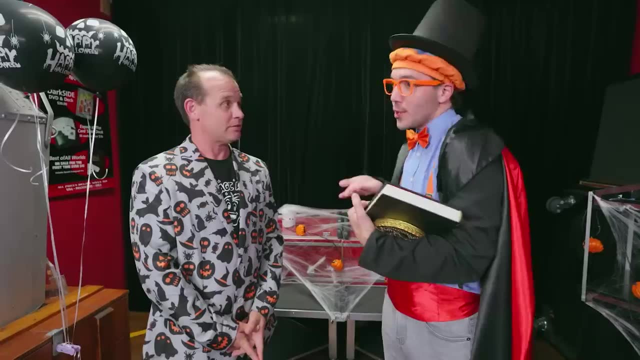 Whoa, so you can learn tricks by reading books. Sure, you can read books. you can get them from the library, or, if you have magic friends, they can all teach each other tricks. That's so awesome. Well, thank you so much for showing us some fun tricks. 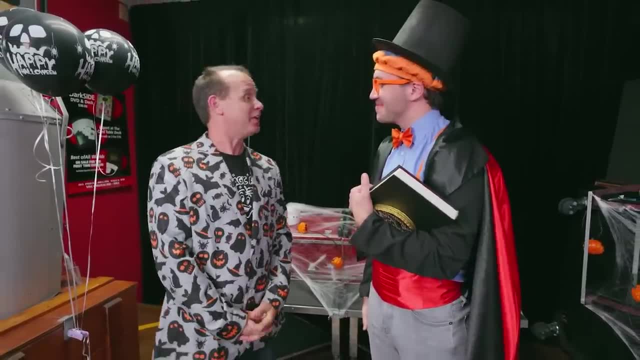 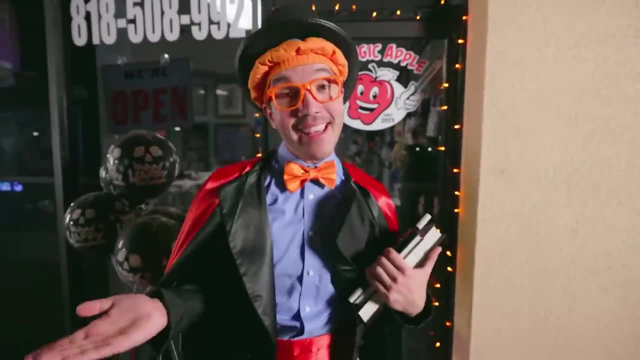 and teaching me how to do some on my own. You're welcome and happy Halloween. Happy Halloween, See you later. Whoa, that was so much fun. Yeah, I had the best day ever with you, learning all about magic tricks.